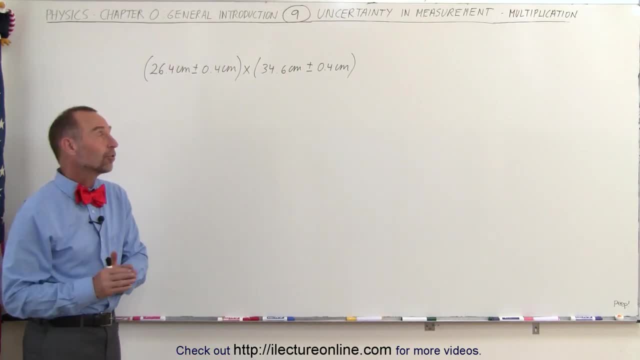 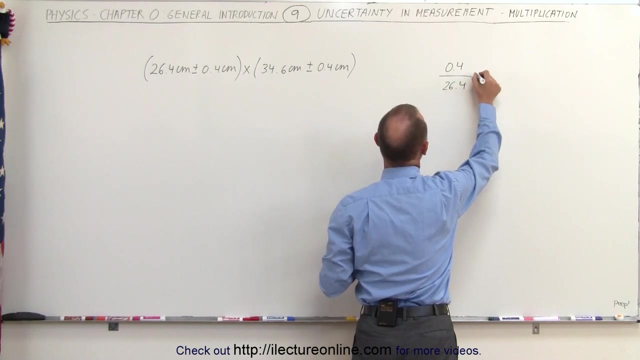 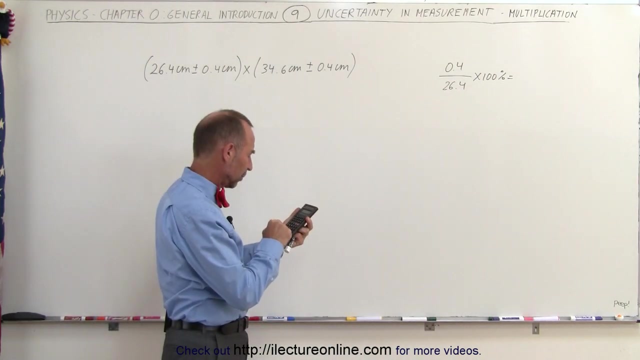 plus or minus 0.4 centimeters. What we need to do first is take these uncertainties and convert them to percentages. What percentage is 0.4 of 26.4?, For example? what we do here is we take 0.4 divided by 26.4 and multiply times 100 percent. All right, using a calculator, 26.4. 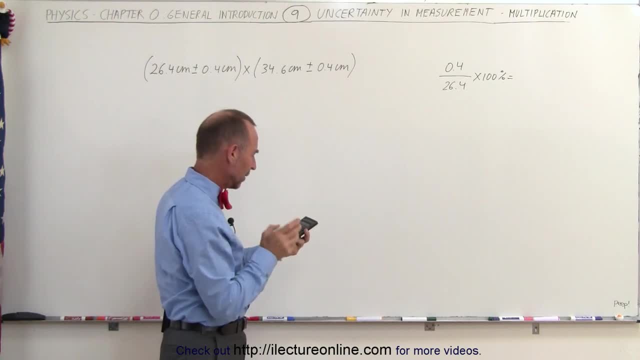 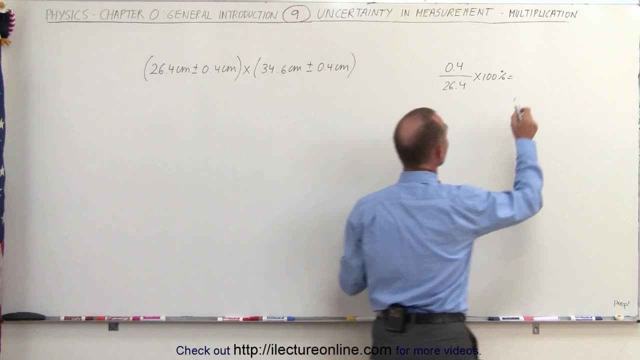 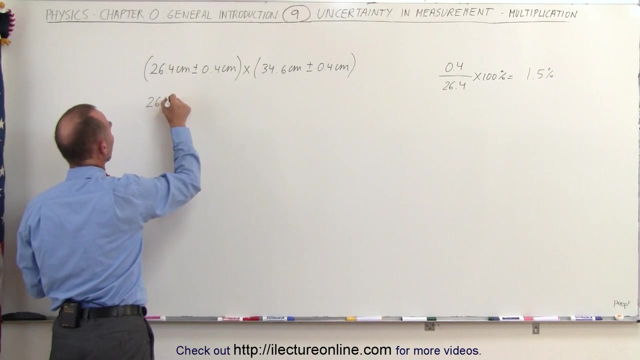 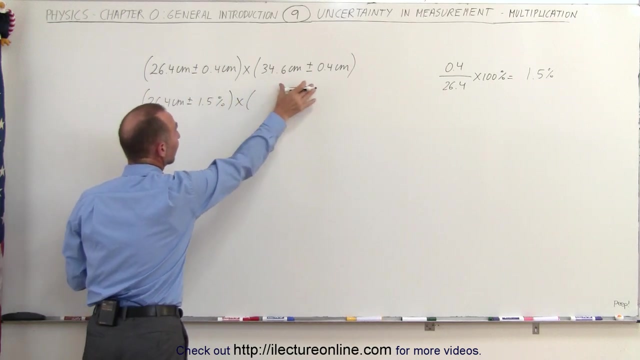 and multiply times 100 percent and we get- oh, let me try that again- 0.4 divided by 26.4, it's about 1.5 percent. So what we're going to do now is rewrite this as 26.4 centimeters plus or minus 1.5 percent, And then we're going to multiply that times this and again. 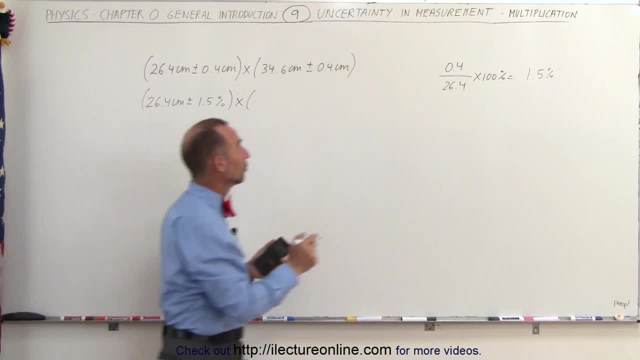 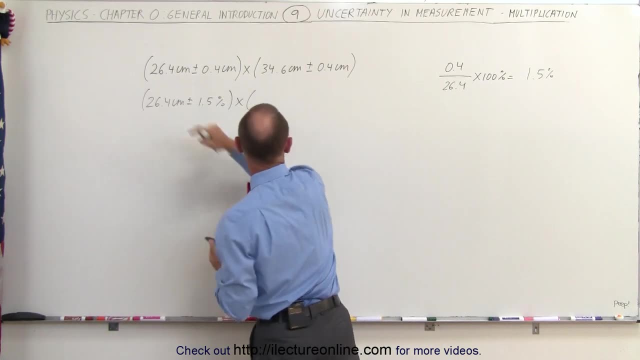 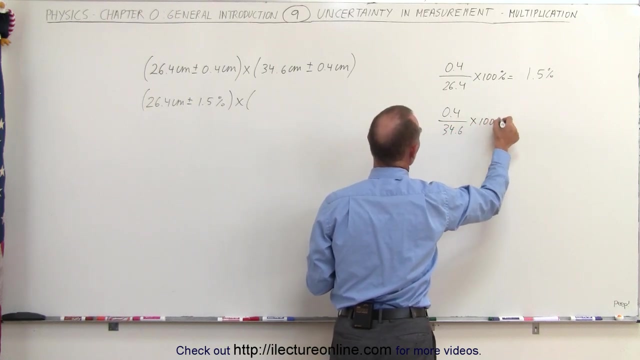 we're going to convert the 0.4 to 2 percent. So notice that this is 0.4 relative to 34.6, is going to be a smaller percent, as 0.4 relative to 26.4.. So we get 0.4 divided by 34.6 times 100 percent. 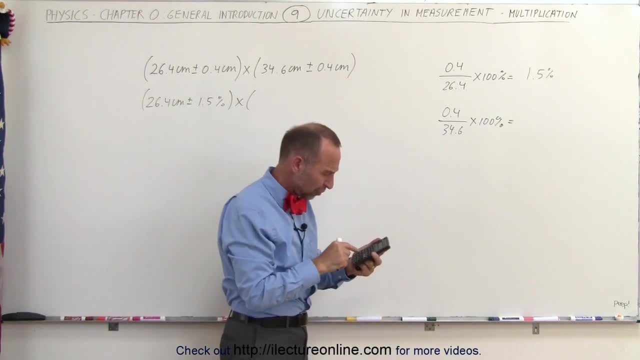 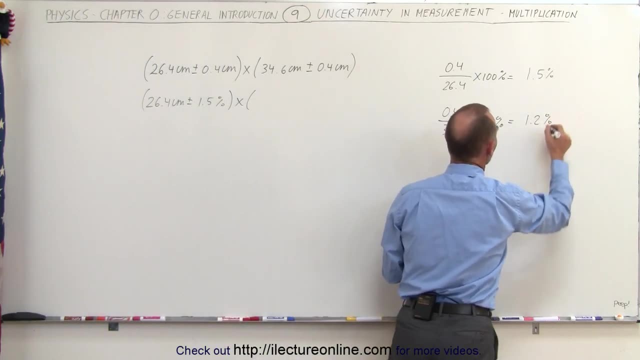 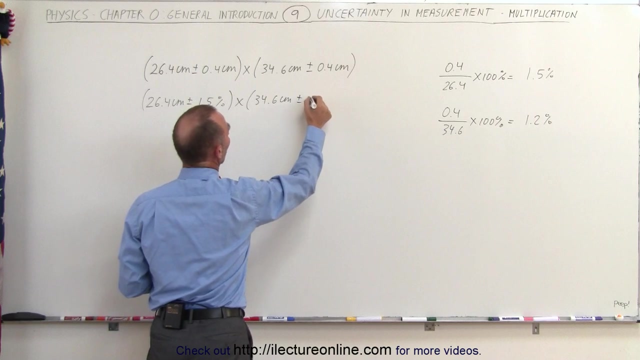 and let's see what that is equal to: 0.4 divided by 34.6.. We get rounded off. that would be 1.2 percent, And then of course we move that over here. so we have 34.6 centimeters plus or minus 1.2 percent Now when we multiply. 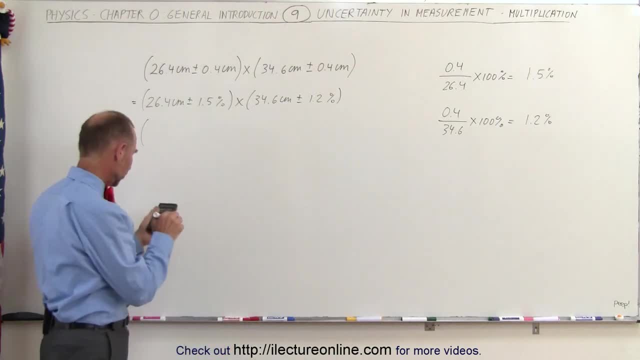 we need to multiply that together, so we have 26.4 times 34.6.. So it gives us 0.44 centimeters squared. Of course it's centimeters times centimeters, with centimeters squared plus or minus. Now what we do here is we add percent uncertainties. So we add 1.5 to 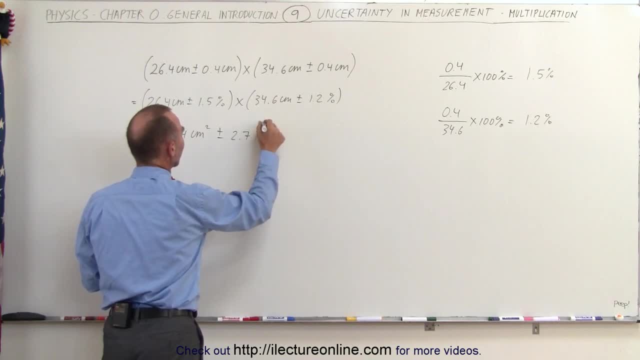 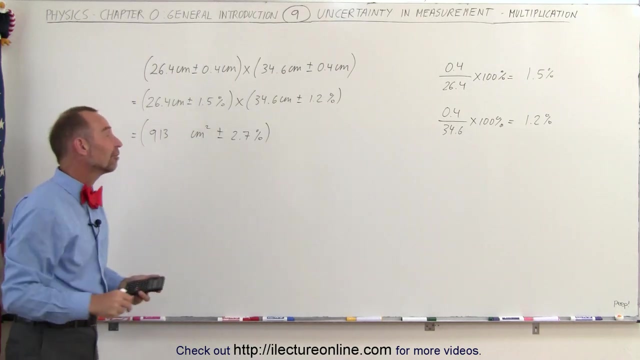 1.2, that gives us 2.7 percent. Now take a look at this, realizing that here we have three significant figures. Here we have three significant figures, So here we should only have three significant figures, which means we really should get rid of the 0.44.. That's really not meaningful.